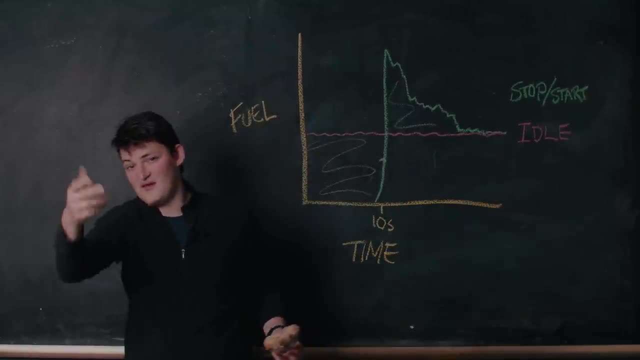 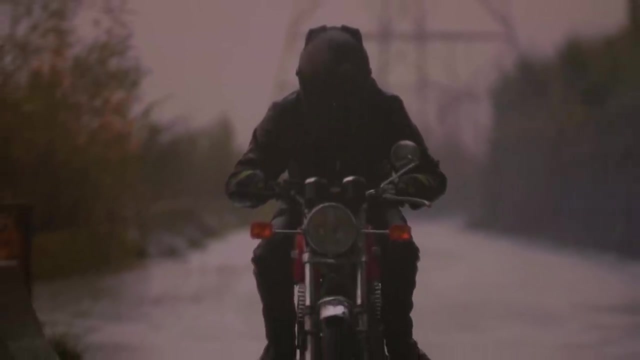 Meaning if you must sit longer than 10 seconds. killing the bike saves gas. Remember that stationary engines get exactly the same energy as a car, So if you're driving a car that's going to be idling for 10 seconds, NPG is a dumpster fire Zero. 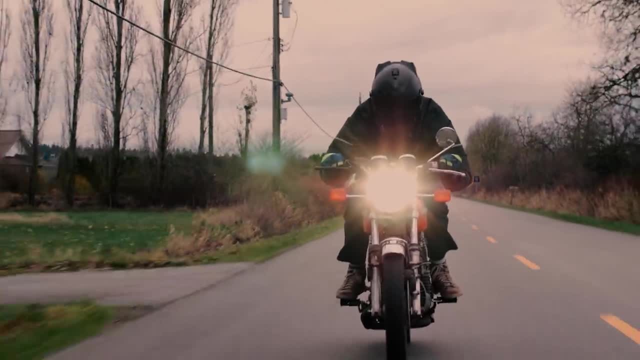 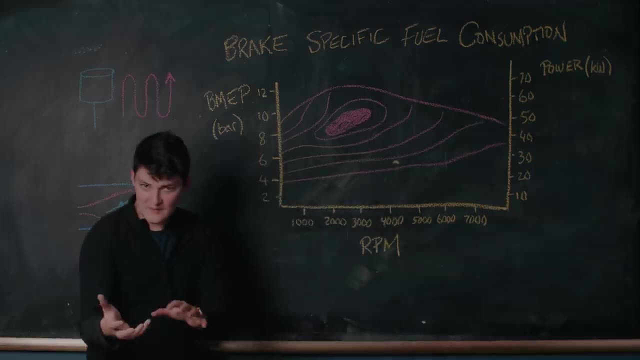 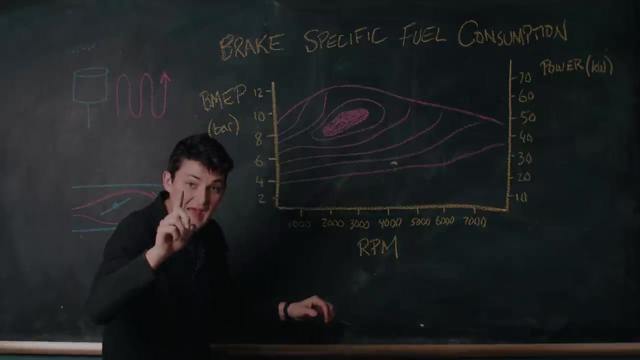 Our rider moves on to chug in 6th gear, But like chugging beer, that's an effective, yet imperfect solution to his problem. See, fuel consumption is a more complicated picture, with the lowest numbers found between 1500 and 3500 RPM at peak engine load. And of course low RPM means fewer rotations. 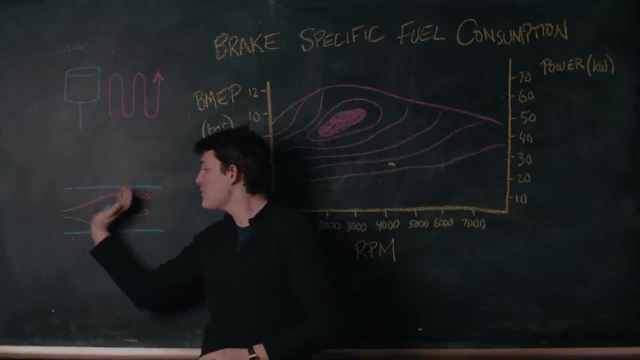 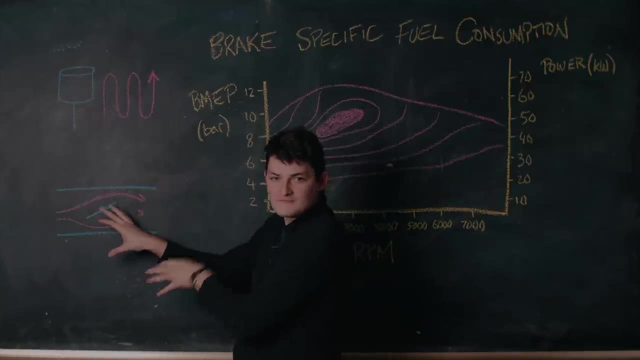 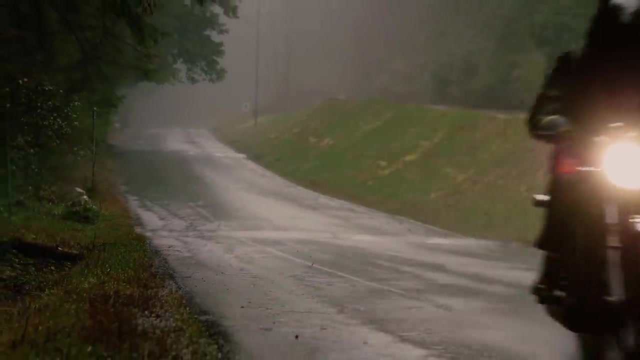 less friction drag, But high engine Engine load means an open, free-flowing throttle valve, less pneumatic drag, Slow and loaded Like a reality TV star, that's how engines go far. Our rider squeezes the most power out of whatever fuel he has left by running 2,500 RPM wide. 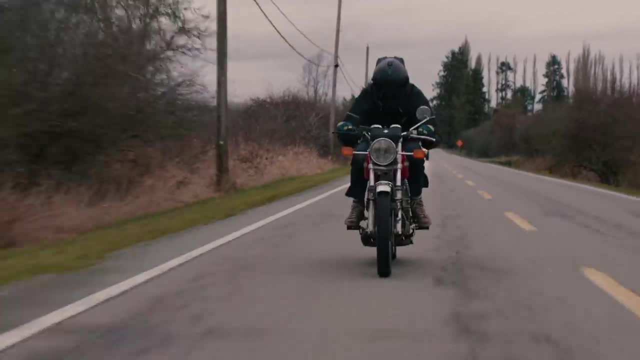 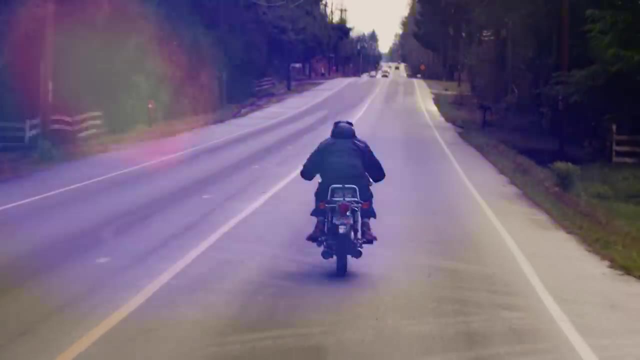 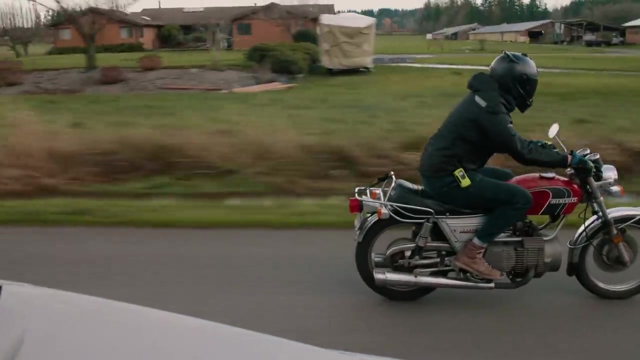 open throttle. But just because it's efficient power doesn't mean you can use it all at once, Not at legal speeds and not without too much wind resistance. Hence the hypermiling technique of pulse and glide. Choose the highest gear, accelerate wide open up to 3,500 RPM, then coast back down and 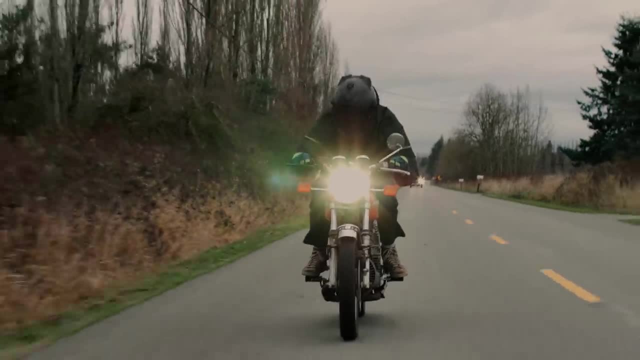 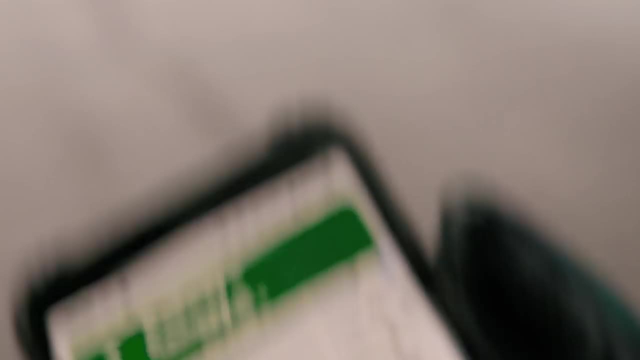 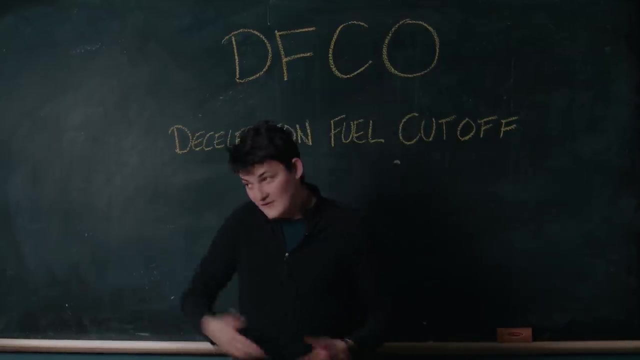 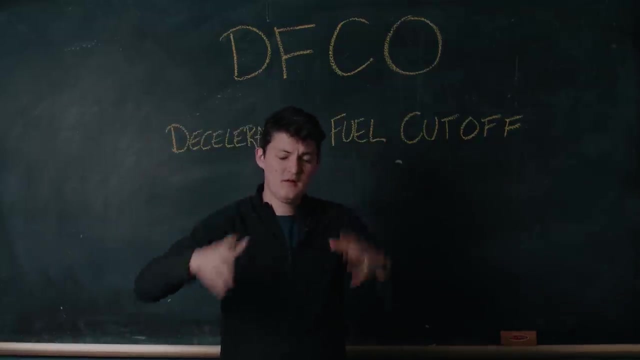 repeat till your destination. Or, as the case will be not, A rider failed to coast correctly. See fuel-injected motorcycles map a deceleration fuel cutoff. In that case, shut the throttle coast in gear. the ECU feeds no fuel. 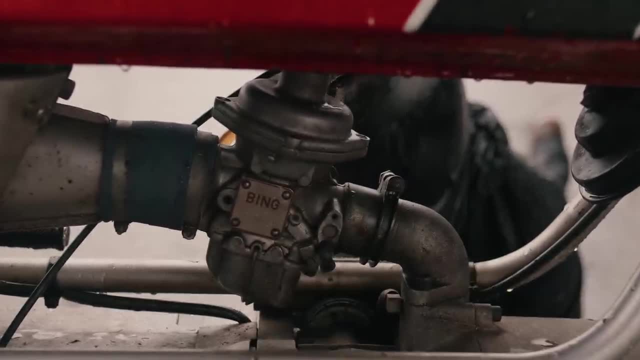 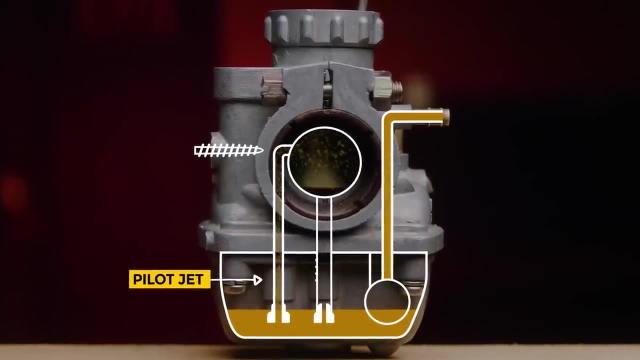 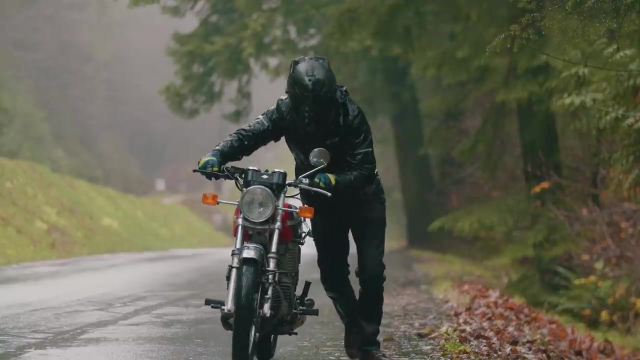 But our rider does not have fuel injection. He has one of these Carburetors always suck gas through the pilot circuit, so in this case better pull the clutch and coast it idle, so at least the carbs suck slowly. Failure to do so has our rider pushing 4.8 kilometers.